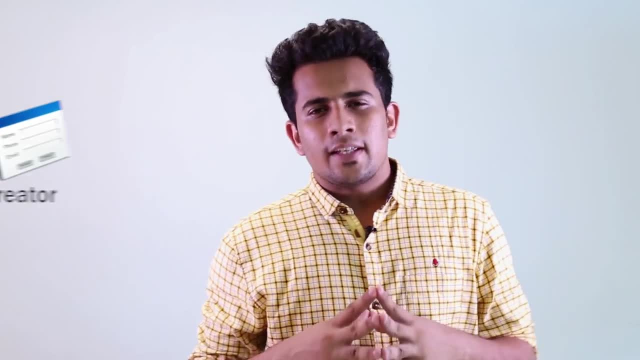 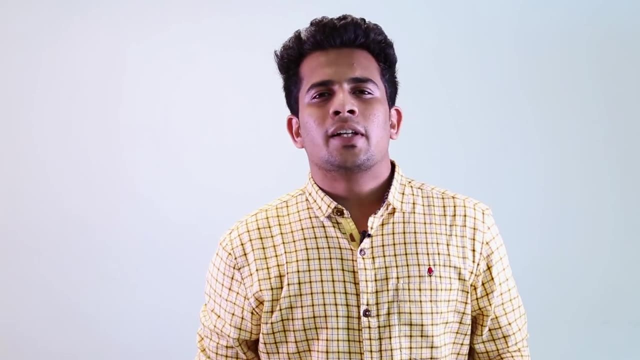 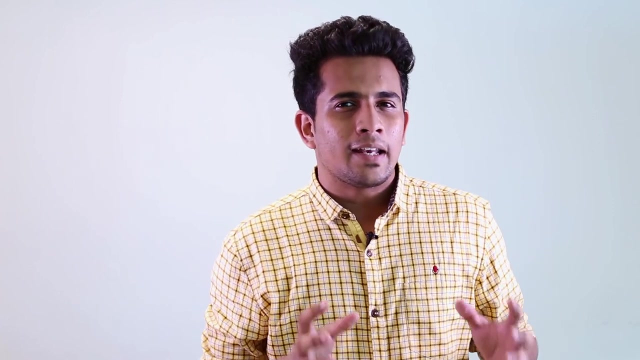 Creator to create the same. Let's take a look at the main features of the application. The application will be able to have a database that will consist of information about the properties, the maintenance staffs and the tenants. It will also help you create records about rental payments. 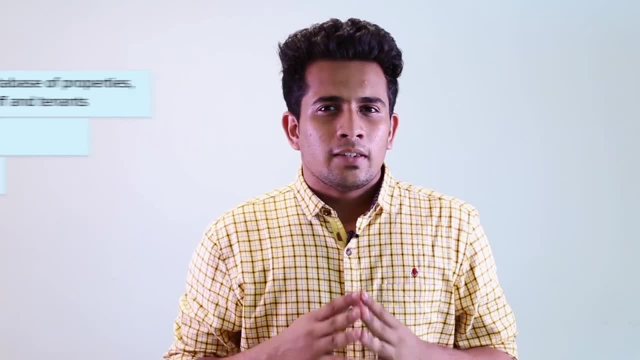 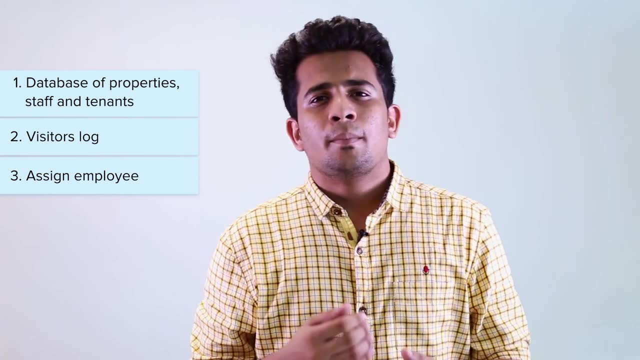 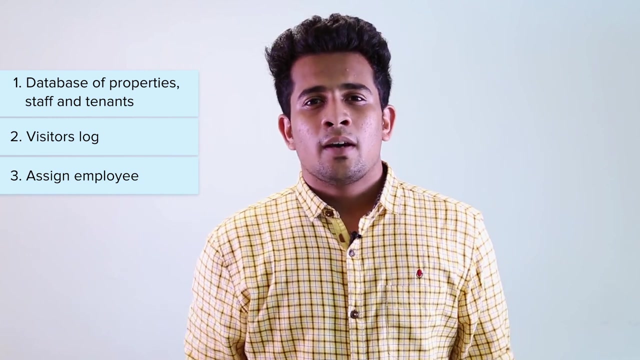 and will also help you create a visitor's log. The application will benefit the manager of these properties the most, because he'll be able to access details about properties, tenants, maintenance staff, visitors- all from the same application. So, without further ado, let's go and make our own property manager application. 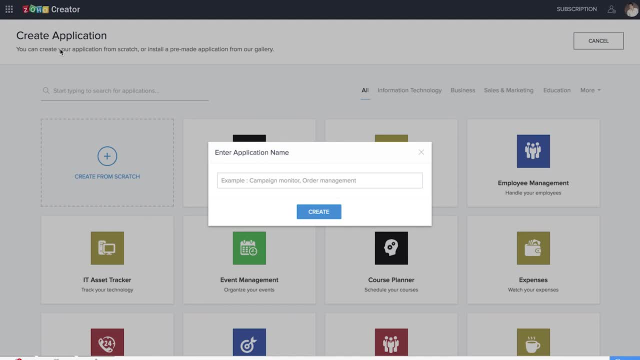 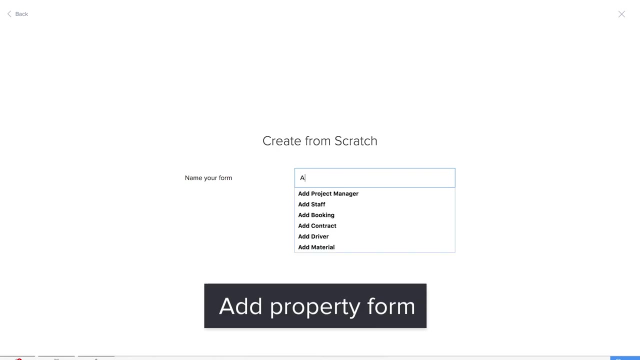 As usual, we are at the create application page of Zoho Creator and we'll be creating an application from scratch. Let's name the application as property manager. We'll be creating the first form, which will be a database of all the properties, So let's call it. 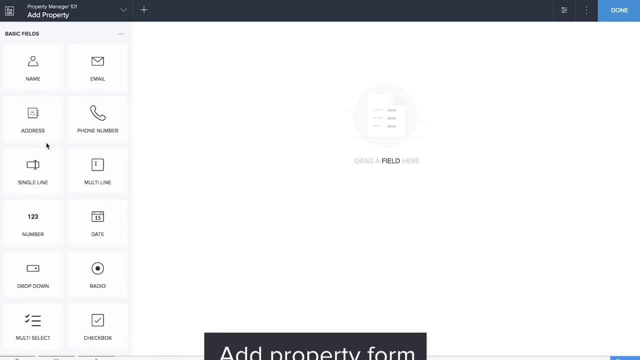 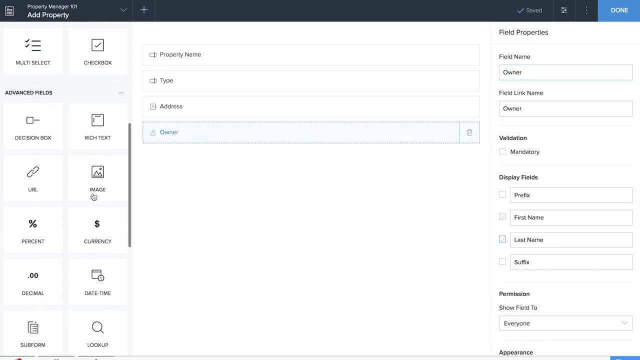 add property. We'll be dragging and dropping a single line field to record the property name, another single line field for property type. We'll also be dragging and dropping the address field, a name field to record the name of the owner and, finally, currency field to record the. 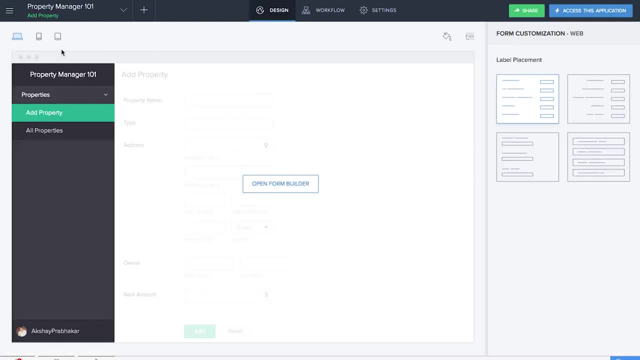 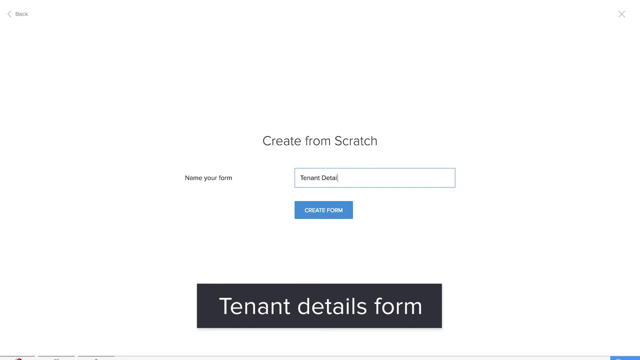 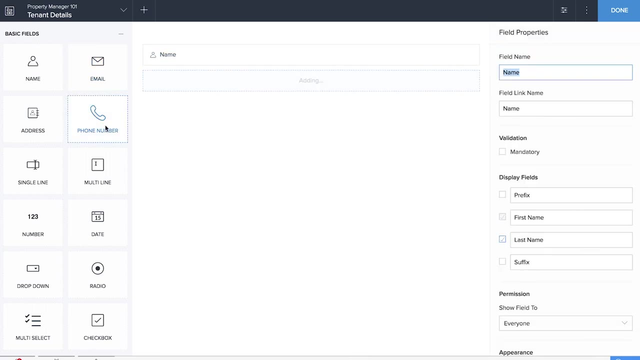 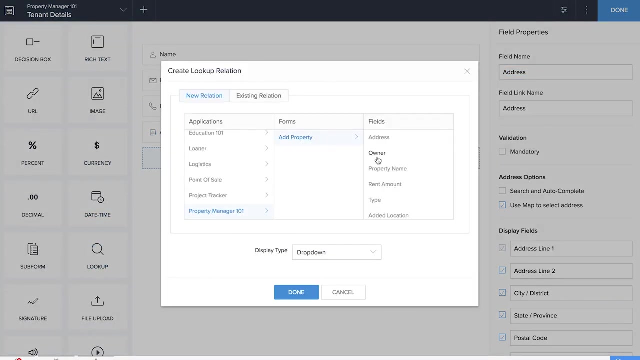 rent amount. Now we are going to create the next form, which is the tenant details form. Here we'll be dragging and dropping fields such as name, phone number and address. We'll also be dragging and dropping a lookup field from the add property form to get the property name. 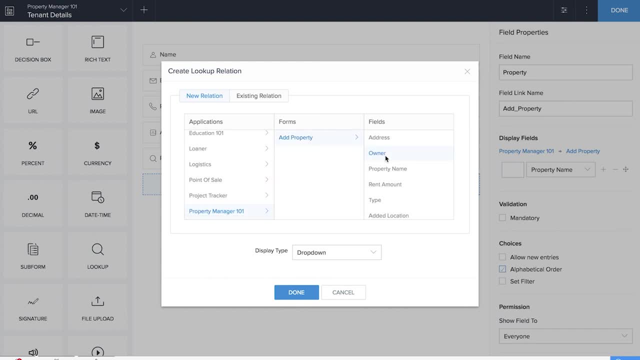 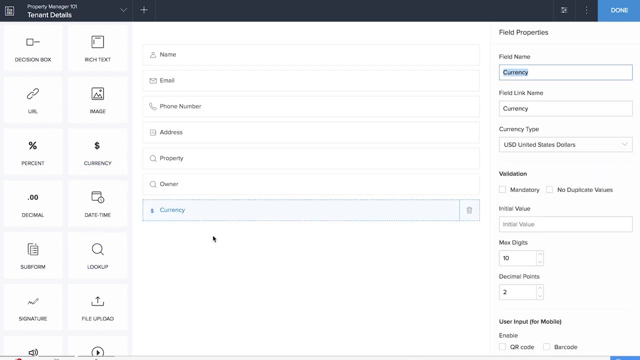 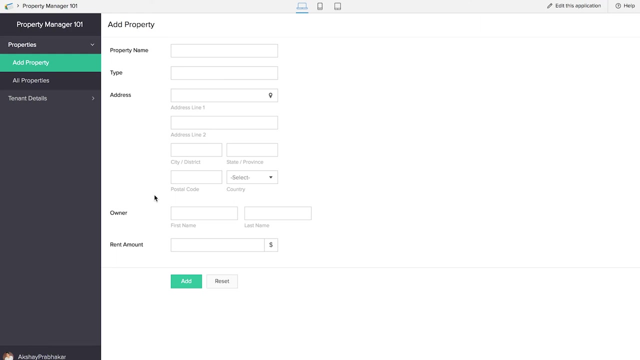 We'll be adding another lookup field for getting details about the owner and, finally, we'll be dragging and dropping a currency field to record the monthly rent. Create the next form, which is the rental payment form. So this form will be able to keep track of rental payments across properties. 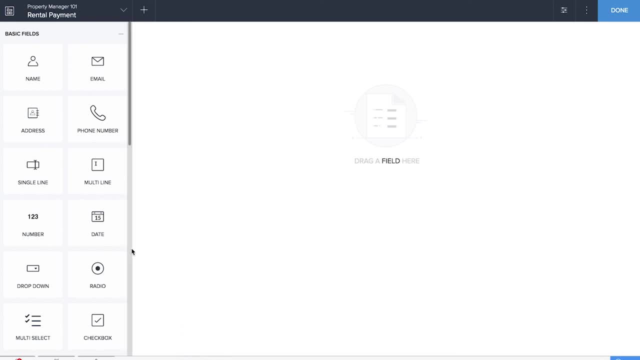 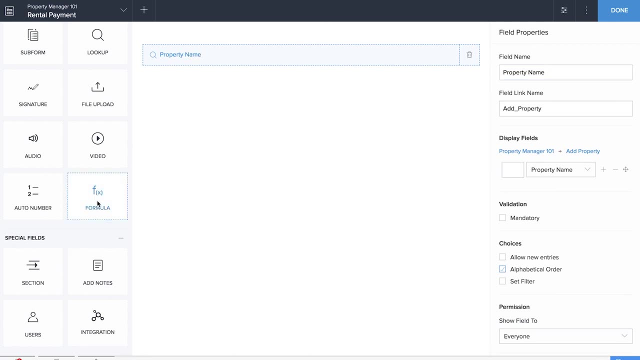 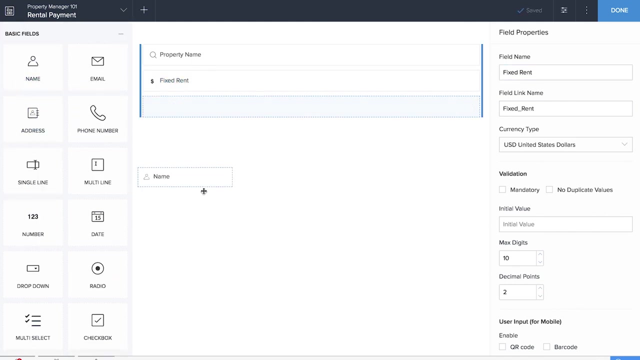 So we'll be dragging and dropping a lookup field for the property name. We'll be dragging and dropping a currency field for fixed rent, a name field for tenant name and also other basic fields such as email and address. We'll be adding a lookup field to get the property name and also other basic fields such as email and address. 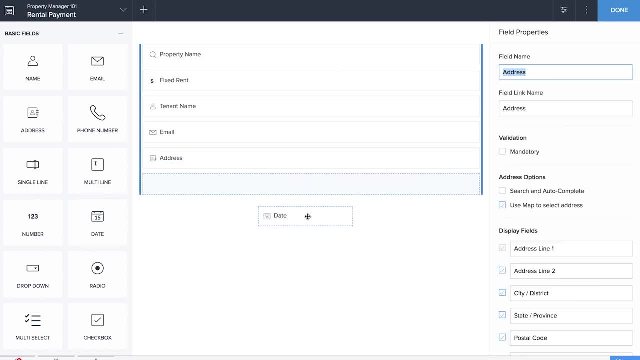 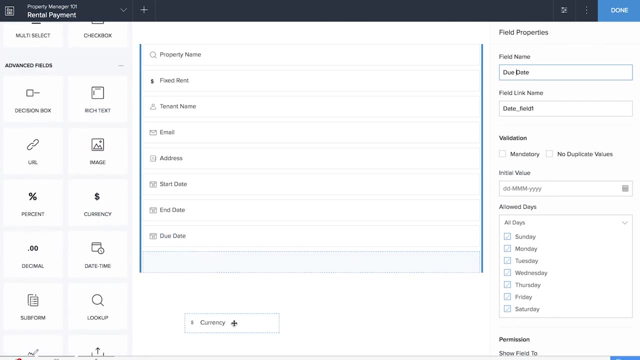 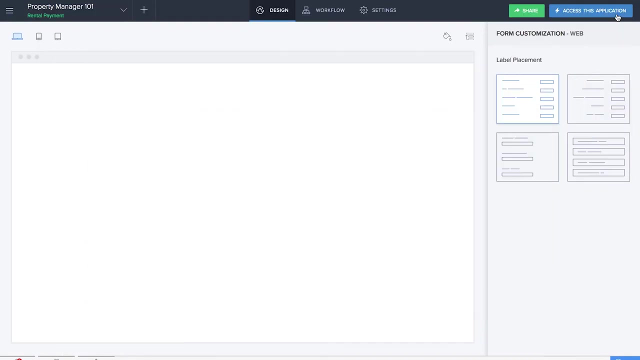 We'll be dragging and dropping two date fields for the end date and due date and finally, we'll be dragging and dropping another currency field which calculates the total amount to be paid. so the rental payment form and report will help you track the rental payments by the tenants based on each and every property. the next form that will do a lot of work for you will be the system reporting field In the drop down menu. you'll just see the system reporting key. just click on12.. Tolerate much and reduce the value of the assetsprech. 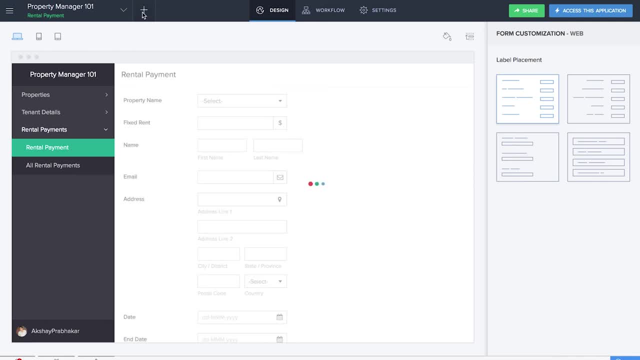 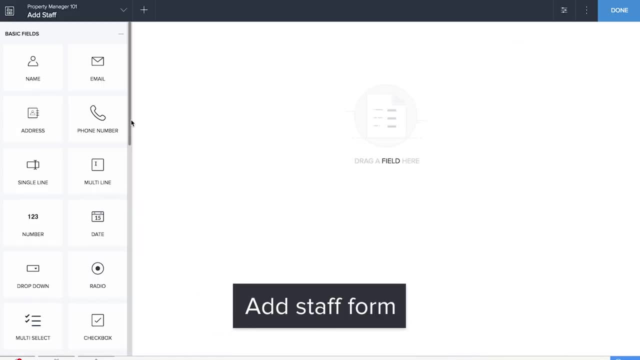 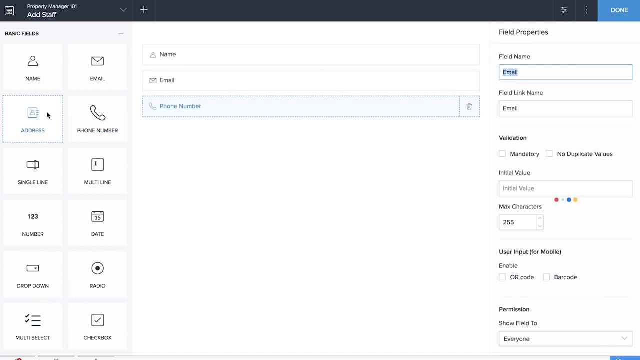 we'll be making is the add staff form, which will act as a database which contains information about all the staffs. we'll be dragging and dropping all the basic fields, such as name, email, phone number and address. will also be dragging and dropping a single line field to 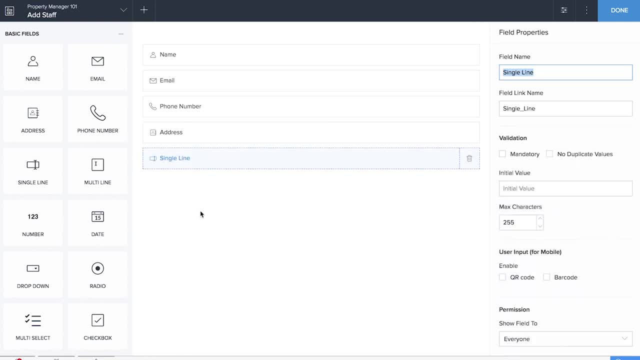 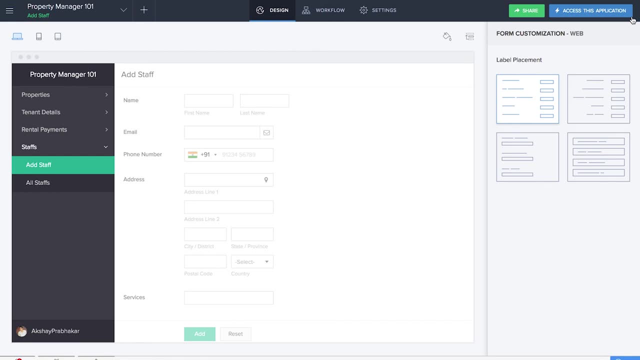 record the services provided by this particular staff, so let's name it as services. now it's important that these staffs are assigned with maintenance work or any kind of work, and its maintenance is one of the most important aspects of property management. so we need an assign maintenance staff form. so 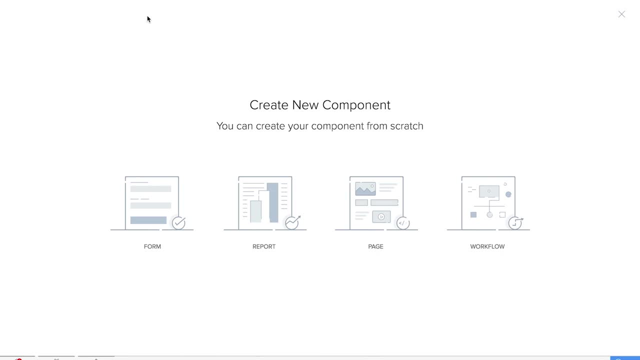 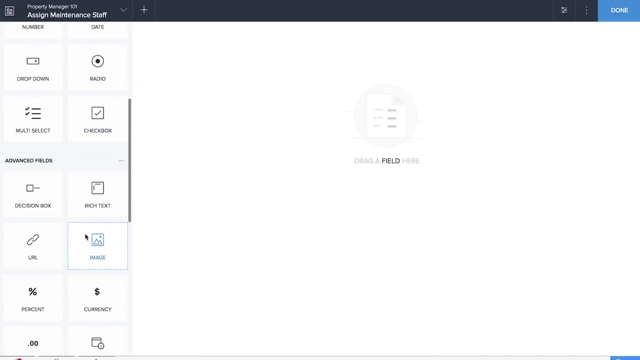 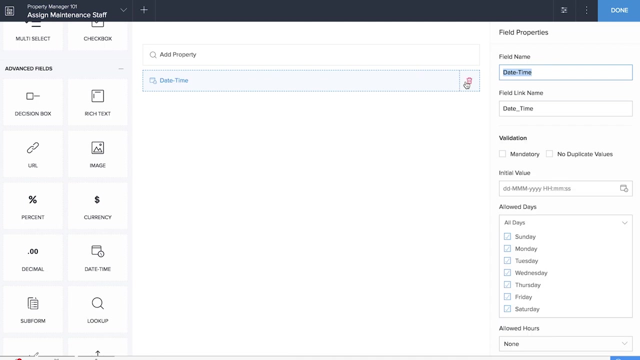 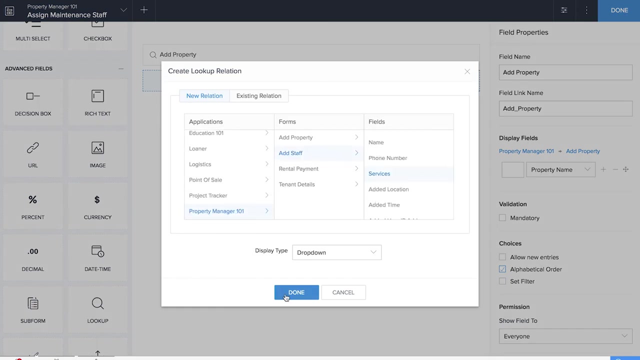 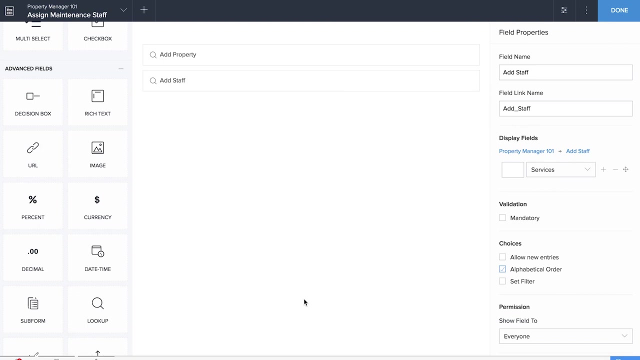 that we'll be able to map the properties with the staff and the services. we'll be dragging and dropping three lookup fields: one is for the property, second one is for the service, the second one is for the service and the third one will be the staff name. 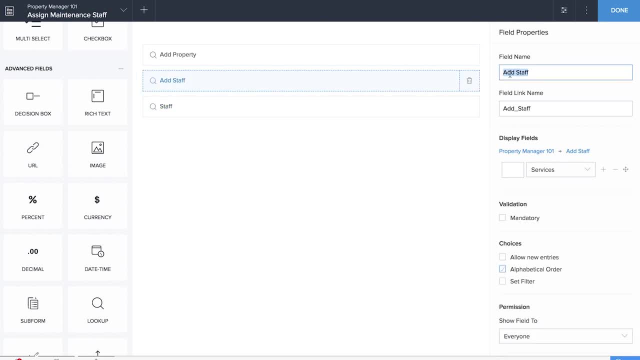 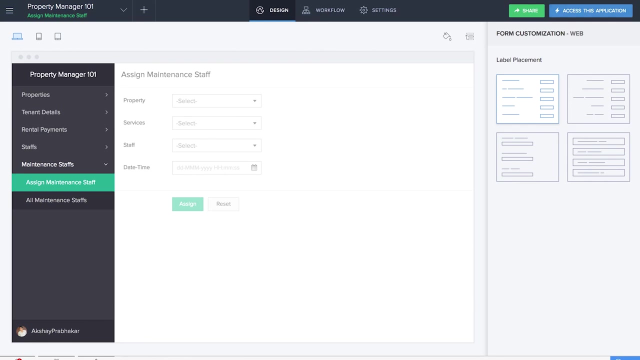 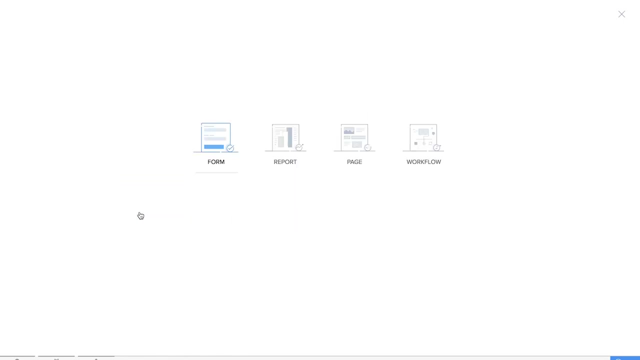 you and dropping a date time field so that the maintenance work is assigned to a particular date and time. now it's time for us to create the final form, which is the visitors form. the next form that we are going to make is the add visitors form. this form will help us keep track of all the visitors entering into each 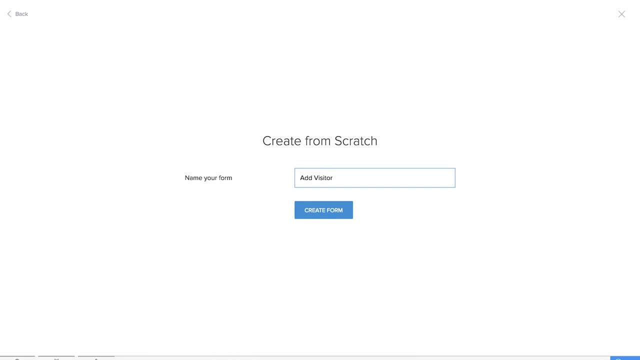 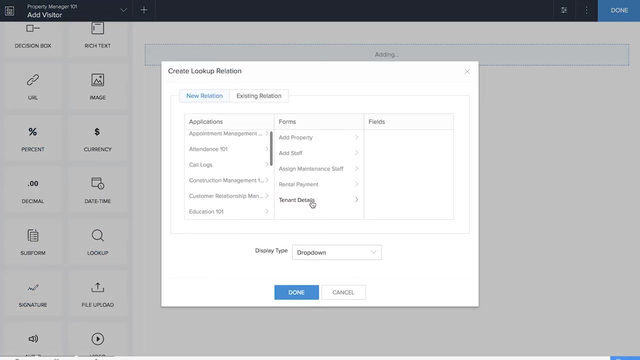 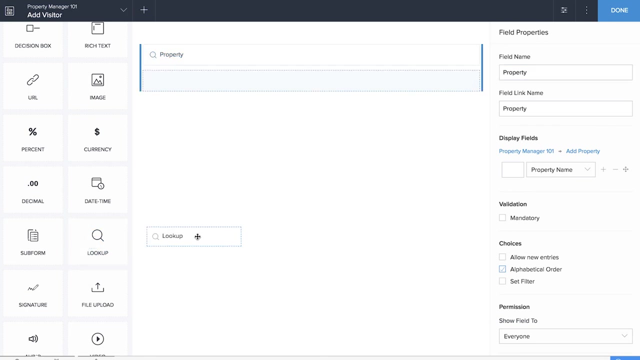 and every property will also have the basic information about them. the first field I will be dragging and dropping is the lookup field to get the property name. we'll be dragging and dropping another lookup field from tenant details and we'll be dragging and dropping another lookup field from tenant details. 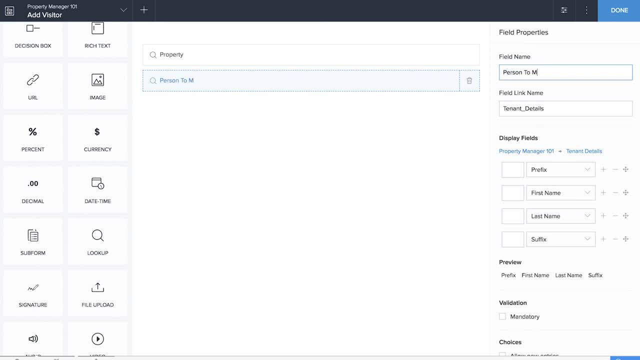 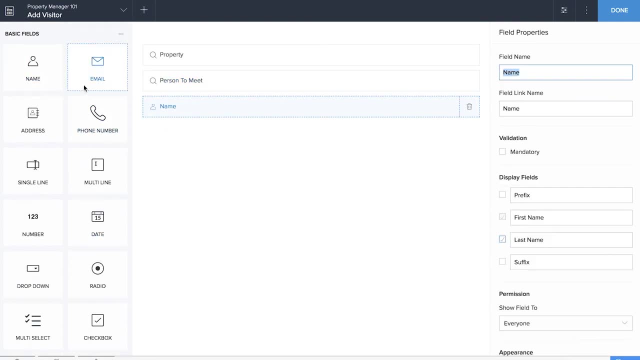 and To get the person to meet. You'll also be dragging and dropping the basic fields such as name, email and phone number. Now we'll be dragging and dropping. now we'll be dragging and dropping a radio field for parking. We'll give yes and no as the two choices here and finally, we'll be dragging and dropping a date time field for. 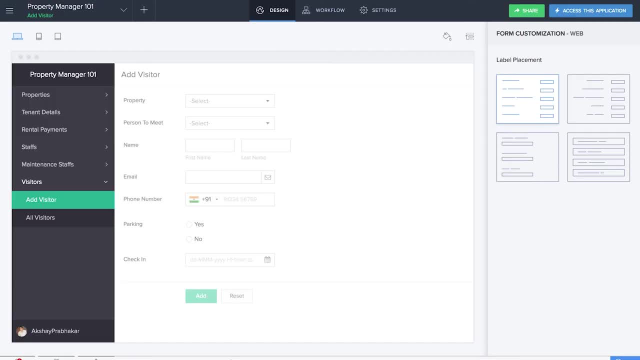 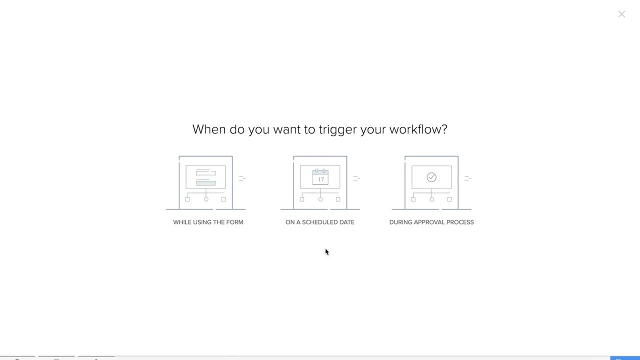 Check-in. Now it's time for us to add all the workflows that will help in automating our application, So we'll be creating the first workflow. it will help us autofill the rental payment details, So we'll name it as autofill Rental payment. Let's click on add new action to create a new action. 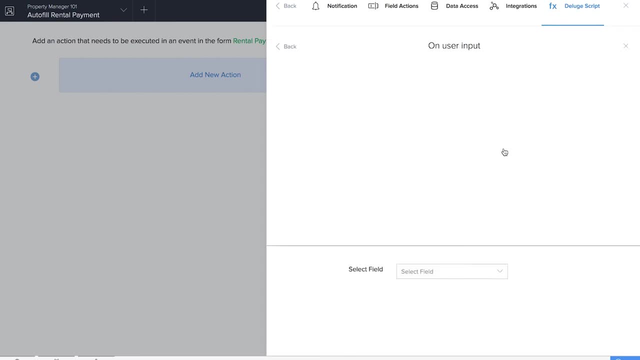 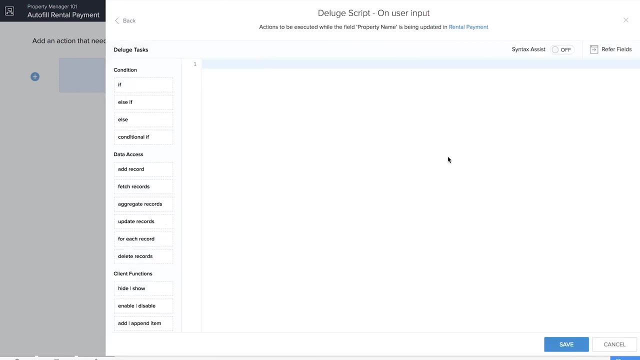 Deluge scripts and we'll be doing it on user input, on the property name field. So let's type our Deluge code, our deluge script, here on user input. So what I've done here is that I've given RDC as the variable and Add tenant is the add tenant form, and since property field or property name field is a lookup, 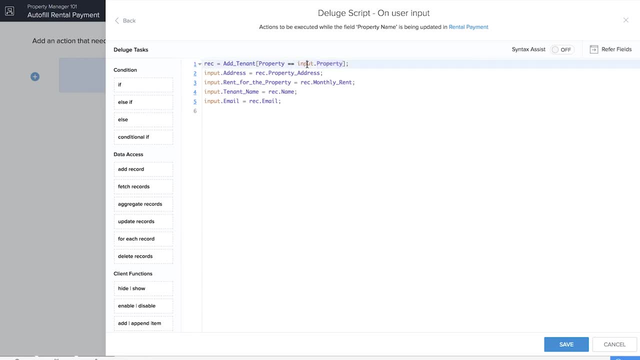 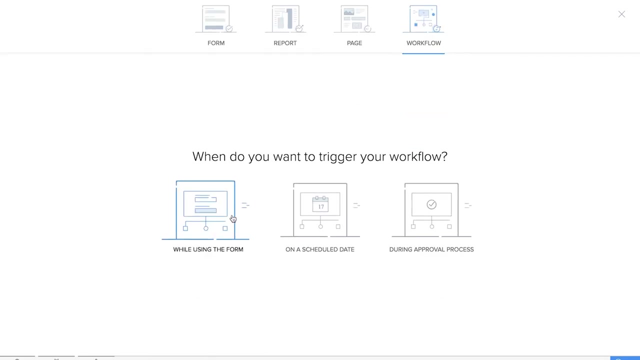 From the property form. we have given it as input- dot property- and we have similarly fetched the details of address, rent, tenant name, email, Etc. from the tenant details form or the add tenant form. So let's click on save Now. the next workflow will help us calculate the rent automatically. 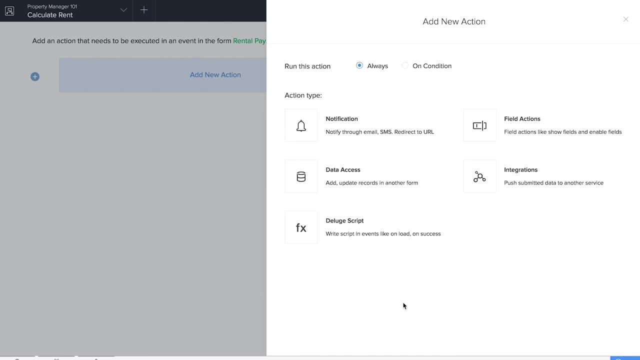 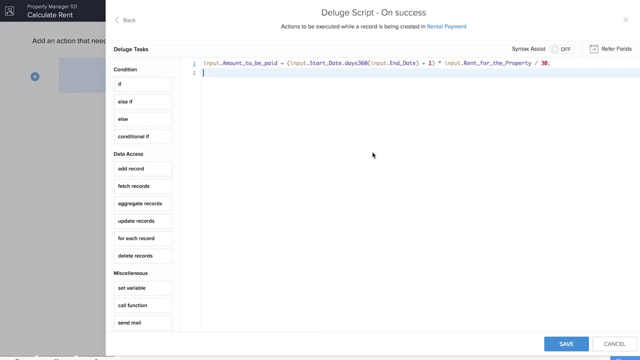 Add new action, Custom action on success. Let's write the deluge script Here. what we've done is: input dot amount to be paid is equal to input dot start date. dot days: 360. input dot end date Is 1 into input dot run for the property. 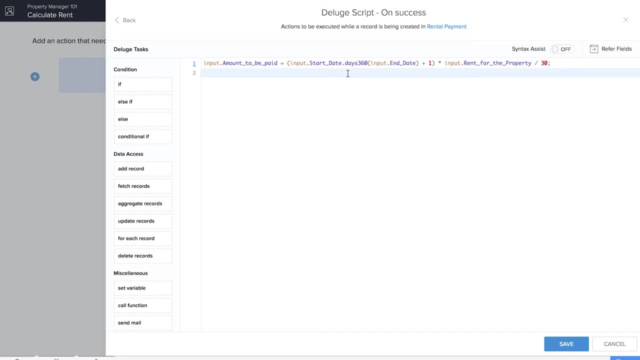 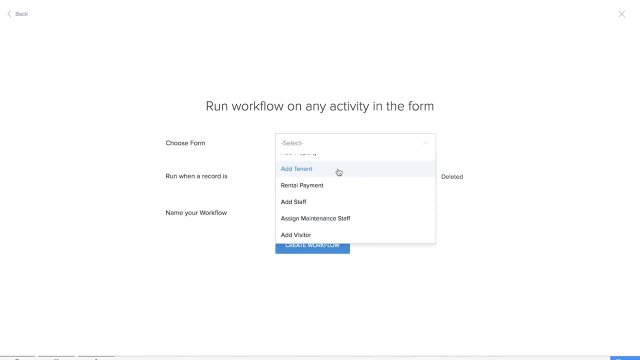 Divided by 30. so we are calculating the amount to be paid by calculating the total number of days, With multiplying it by the rent for the property, and save the workflow, Workflow while using the form Tenant details or add tenant. so it is important to notice that we have done a similar workflow for rental payments. 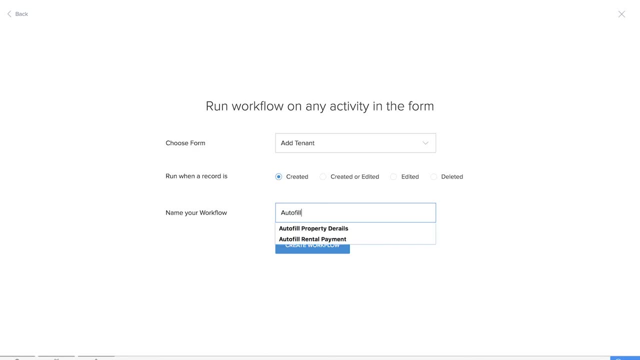 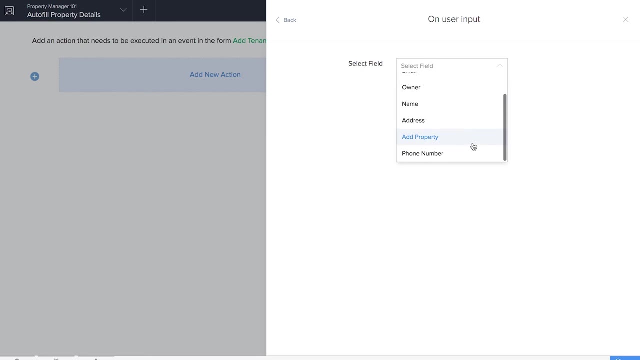 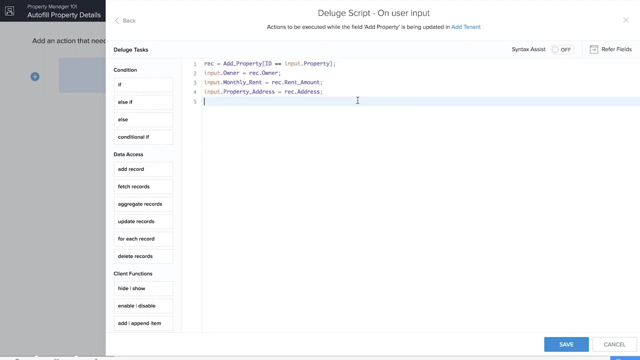 we'll name the workflow as autofill property details and We'll add a new action on user input and in the add property field We'll write the deluge script over here. We'll write the deluge script over here. this is similar to what we have done in the rental payments form workflow, as we have given REC as the variable and 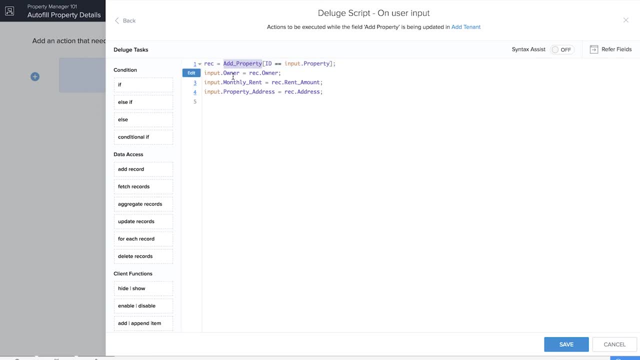 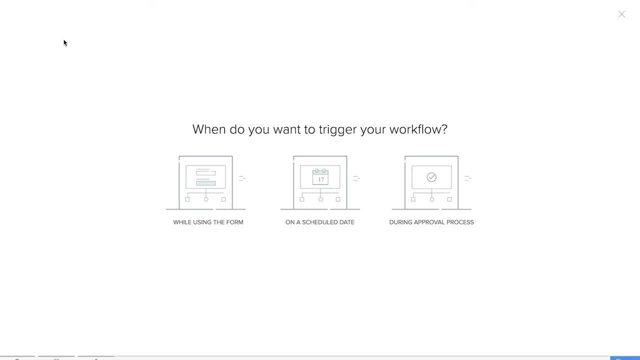 We are fetching details from the add property form. We have also fetching details such as owner, monthly rent and property address. Let's save the workflow. So the next workflow that we are going to create is To automatically fill the check-in time in the visitors form. So we'll click it while using the form. 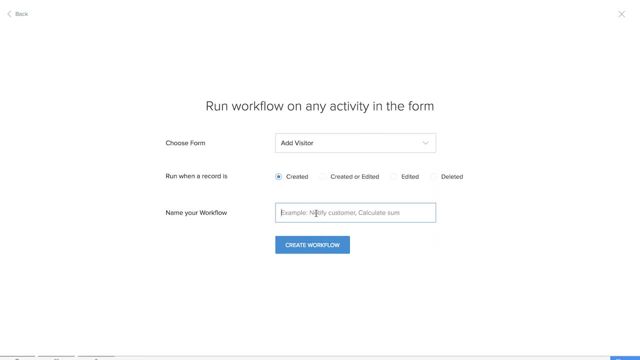 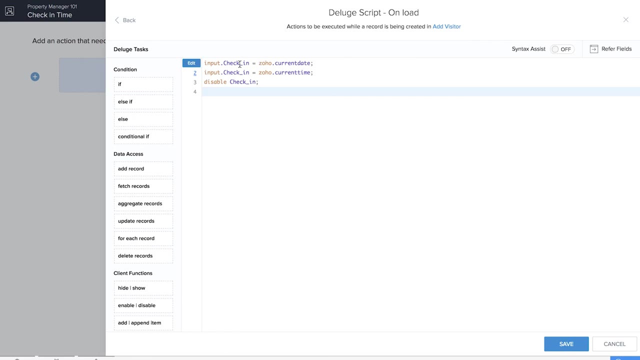 We'll choose the form as add visitor and we'll name the workflow as check-in. We'll add a new action on load. We'll write the deluge script. So we have given input dot check-in as Zoho current date and Zoho current time and you can't. you've disabled the check-in field here. 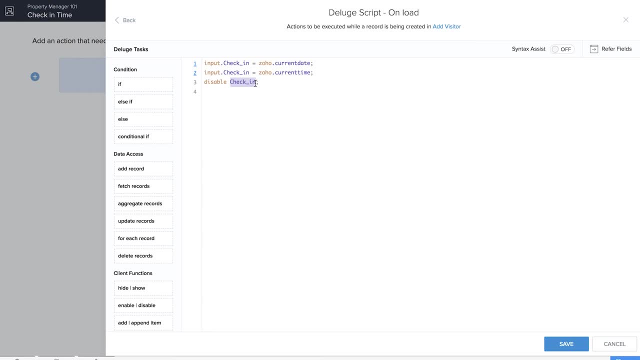 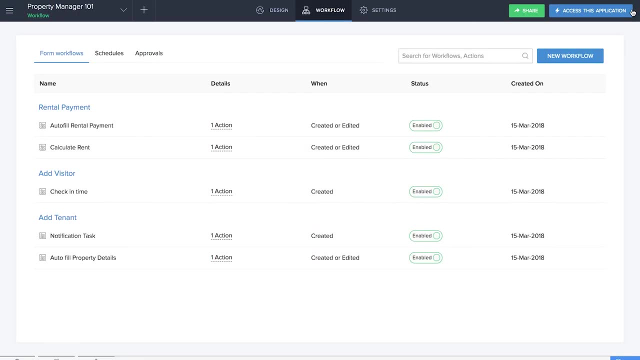 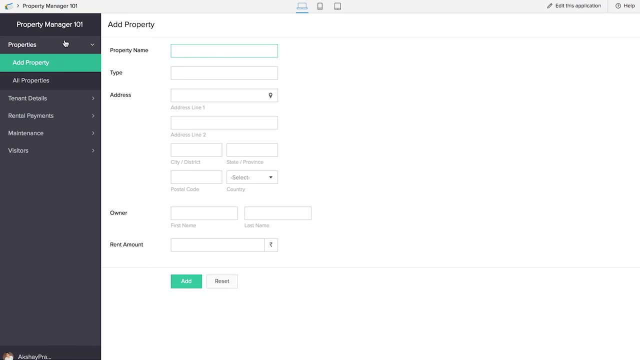 So that nobody will be able to change it or manipulate the details in the add visitor form. so let's click on save and save the workflow. so we are done creating all over flows. now it's time for us to test our application. let's add details into the add property form. 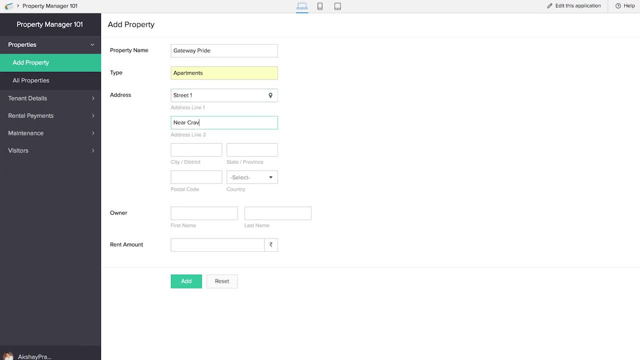 you. so I have given an address and property name and type over here and we'll be giving the owner name as well. we'll be giving one rent about as well into the tenant details form. we'll give a name and an email ID and since we did an out of fill workflow, it is important that if 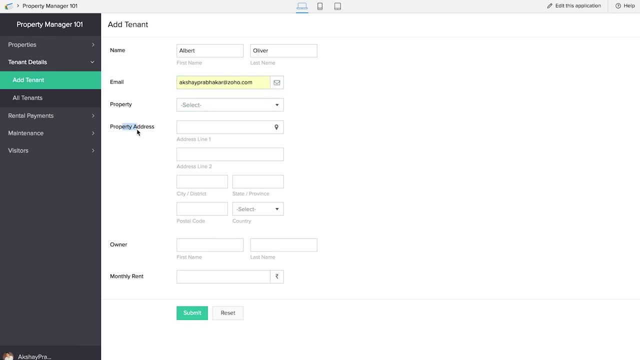 we click on one of the properties, the rest of the details, such as property address, owner, monthly rent, etc. should automatically appear here in the add tenant form, so it is automatically appearing here. if we take another property, the details regarding that property will come over here in the add an inform. now it's time for us to check the rental payments. 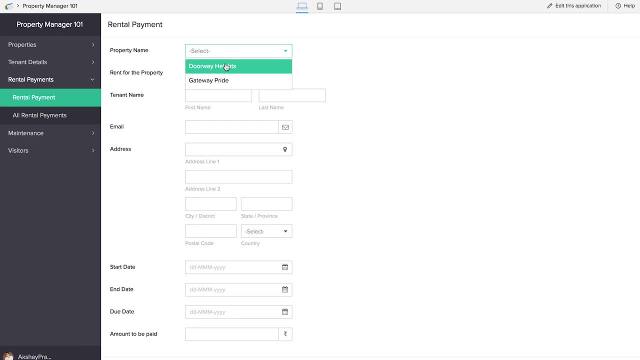 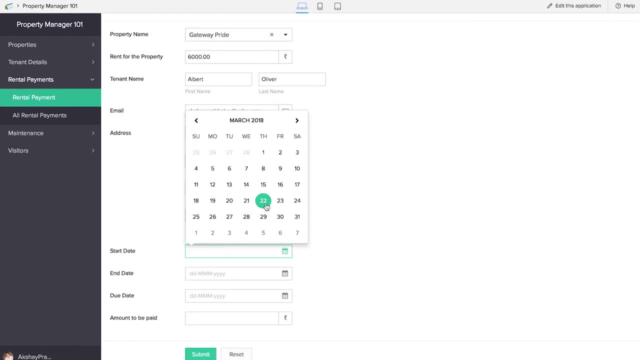 option. click on the property name and all the information have automatically appeared here. we give the start date as 22 March and end date as 22 May. due date is also 22 May. due date is also. you can see here that the amount to be paid have automatically appeared here because of the workflow we did. the 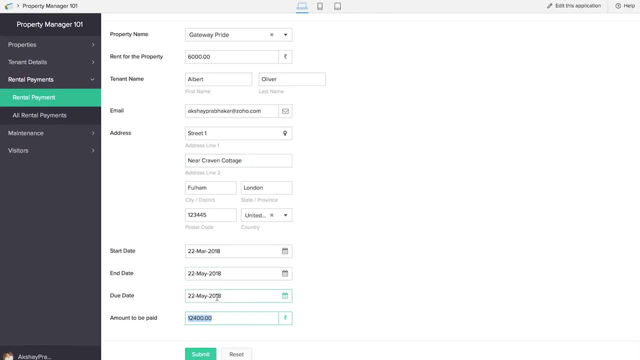 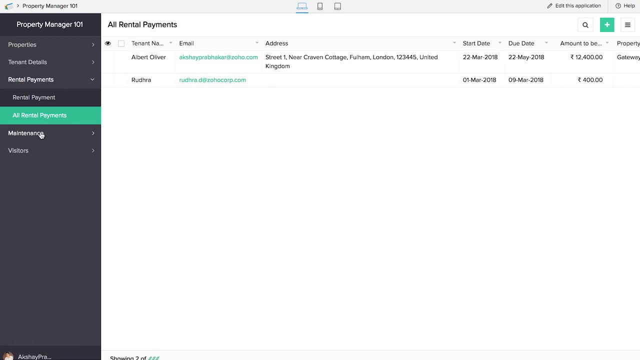 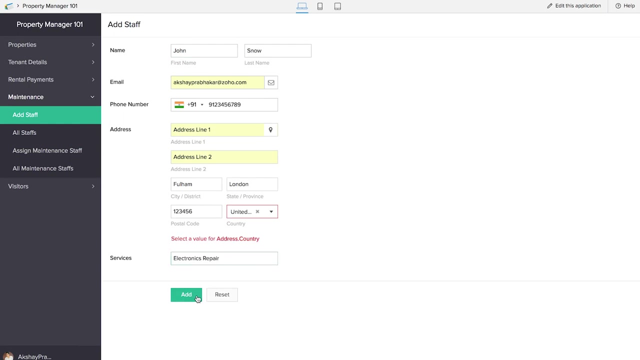 rental payment is automatically calculated based on the start date, end date and the due date. so let's click on submit and that detail will appear here in the all rental payments report. now it's time for us to add staffs. added all the necessary details to the add staff form and we'll be able to see this in the add staff report now. 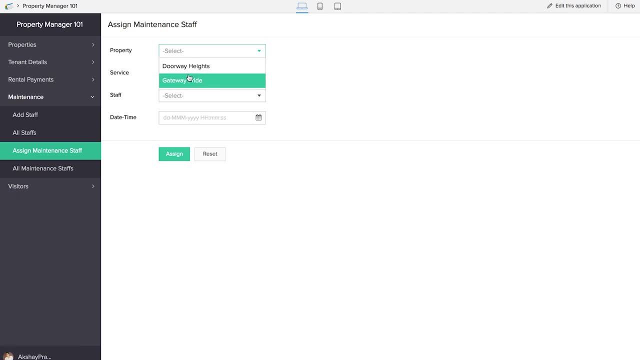 it's time for us to assign a maintenance staff to a particular property. we have given a staff and we will be also giving the service and we'll schedule it for the next day. and if we click on assign, the maintenance staff has been assigned successfully and a mail has been triggered to the staff notifying him. 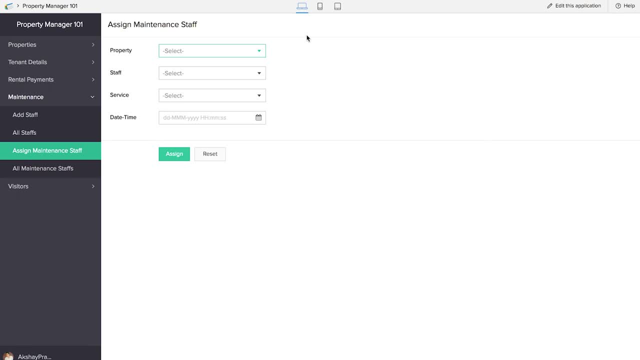 about maintenance project that has been assigned to him. so we're going to take a look at the final part of our application, which is the add visitor form. we'll be adding a visitor person to meet, be giving an email ID as well, choice of parking, number of visitors accompanying him, and the check-in time is automatically. 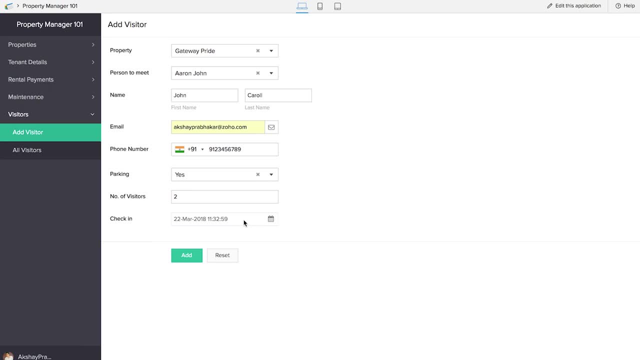 appearing here because of the workflow check-in time that we did during the workflow process. so if we click on add, we'll be able to see all this information in the all visitors form. our property manager 101 has successfully hit all the objectives, like having a database of properties tenants.